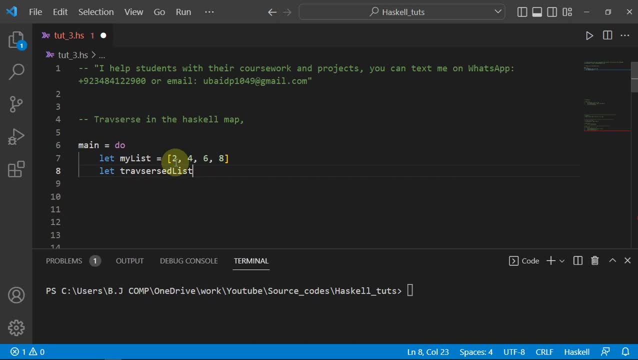 travel list, and here I will use the map function. and if you are enrolled in any Masters of Bachelor program, you can contact me on this WhatsApp or this mail to discuss about your coursework or projects you are working on. all right, okay, let's use the map function here and map function. 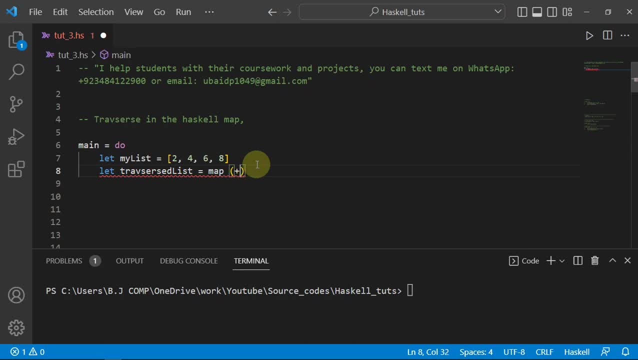 let's have two arguments in which first will be the operation which we want to do on our list, elements one by one, and the second will be our list. so in this case I will just pass my list, which is this variable which has the list, and so this map function. what it will do is 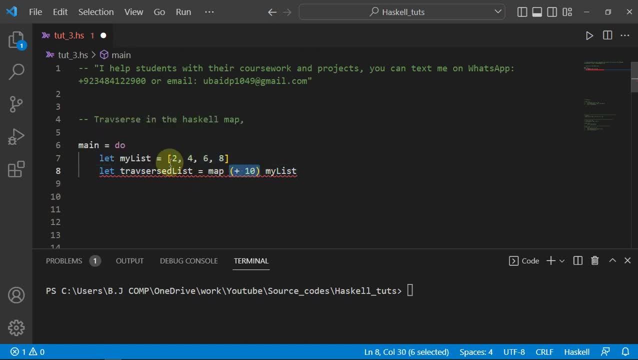 just do this operation on this list one by one. so in Haskell is just this one line of code: um, we just do that right and then I can just print this troubles list and I hope it will works. so let's just run this program and I have set up this. 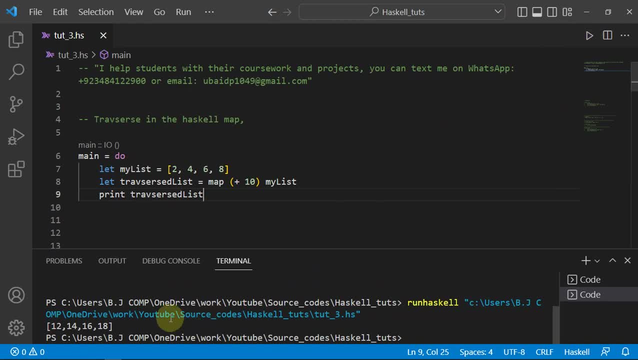 environment with the code runner extension and you can see, we have just, uh, made this operation success, success, successfully with this map function, right, and the operation was very simple: just adding 10 to 8 element in our list, right, and we got 12, because 10 plus 2 is equal to 12 and 14 and so on. so this: 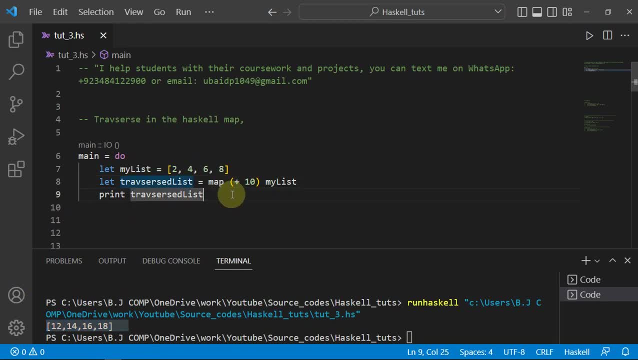 is how you can traverse a list or any sequence in the haskell, and that's it for this video. i will see you in the next one. thanks,